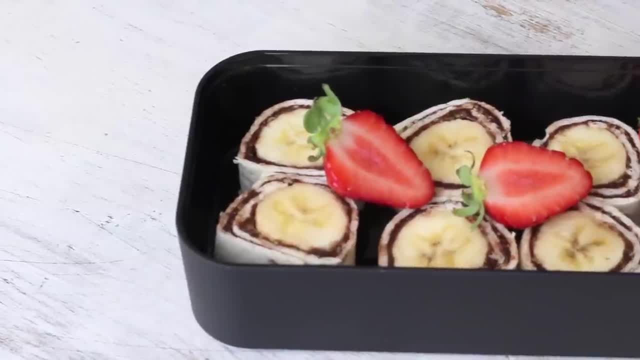 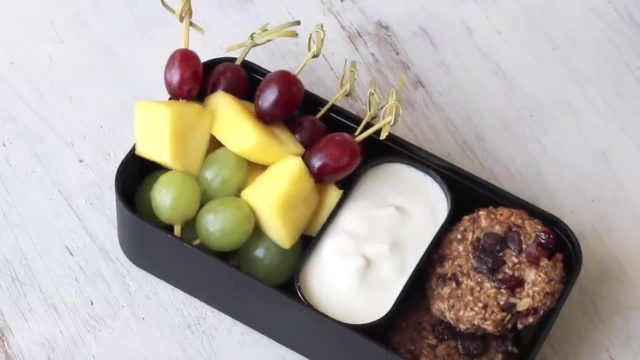 fiber, healthy fats and protein from the nuts that are in that chocolate spread. You don't have to be a kid to enjoy this lunch. that's a guarantee. Now on to making the snacks, which is a fruit and yogurt dip with some homemade cookies. I made these fruit skewers using fresh grapes and 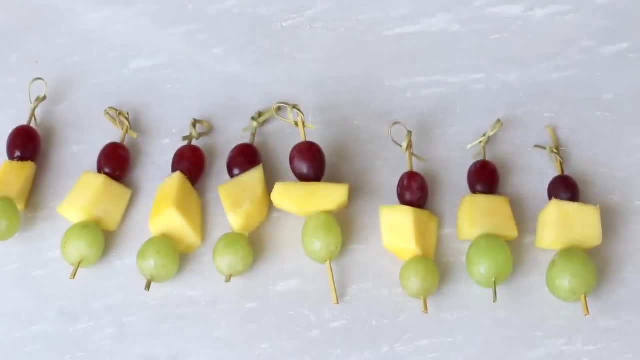 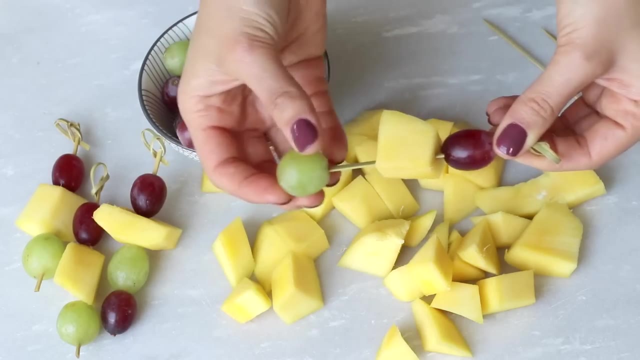 mango, but of course you can use any fruits that you have on hand After you've prepared the fruits and placed them on the skewers. I also chose to cut off the ends, so there's no sharp bits going into the lunch box. Then, on the side, I poured in some calcium. 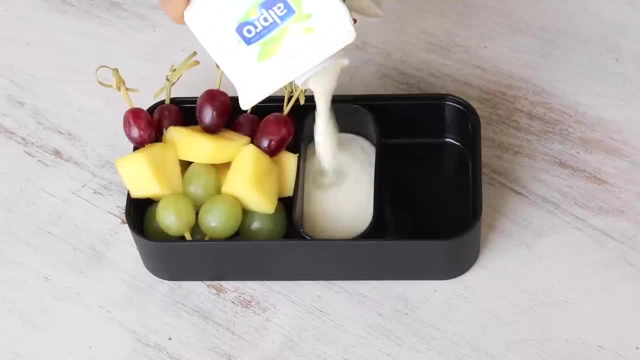 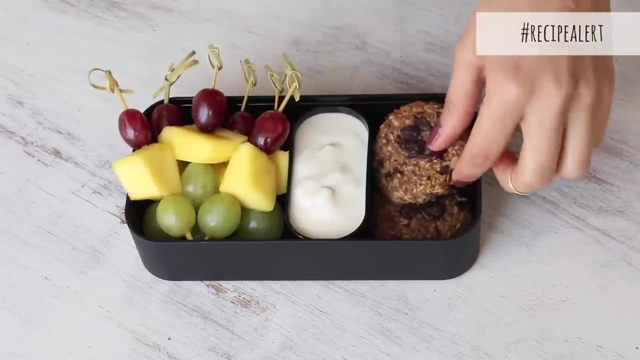 fortified plant-based yogurt. Here I used an unsweetened soy yogurt and this can serve as a dip for those fruit skewers. I also included these one bowl peanut butter and chocolate cookies. I've mentioned these in a previous video and I absolutely love making them because they have no. 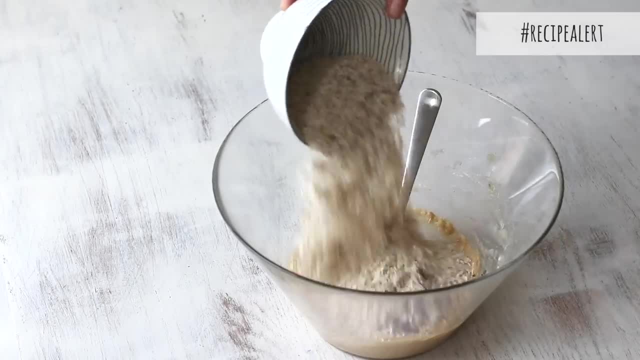 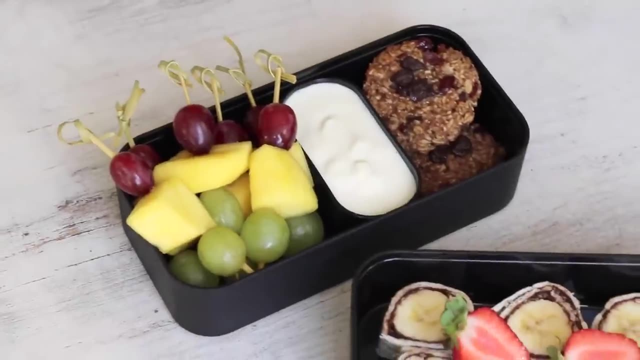 added sugar or oil, and they can be made easily and in one bite, So I'm going to make these in a bowl. It takes only 15 minutes to make from start to finish, so you can batch make this on the weekends to enjoy as a snack throughout the week. And that's it for lunch box number one. 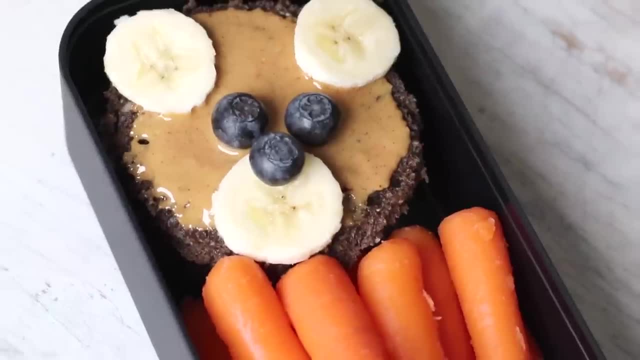 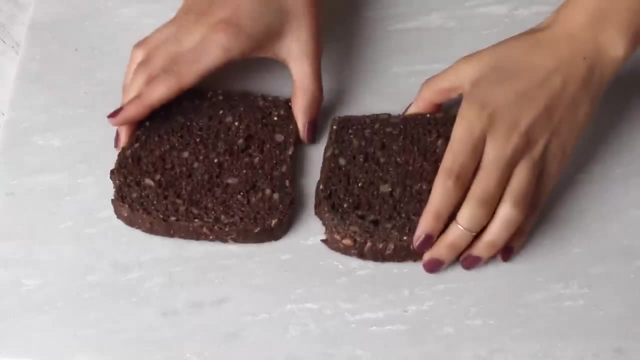 Moving on to lunch box number two, we begin by making this super adorable nut butter and fruit bear sandwich To make. start off with two pieces of whole grain bread and you can use a cup or cookie cutter to cut circles out of the bread. 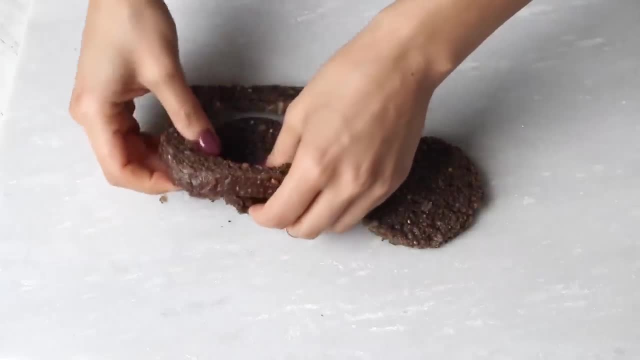 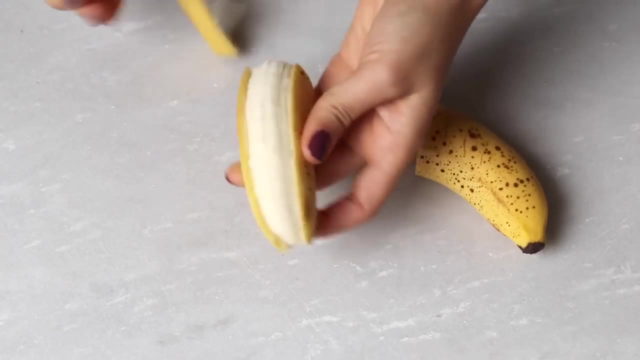 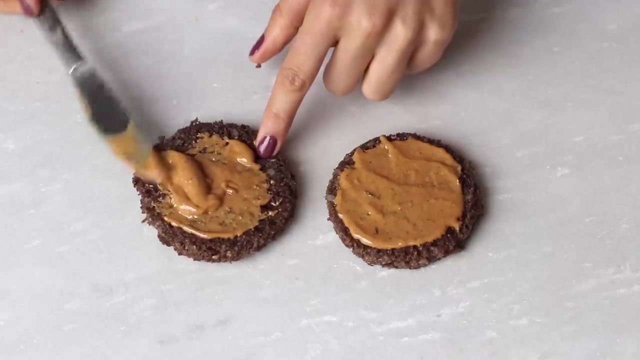 Then, using about half of a ripe banana, peel and slice some banana coins. After you've spread some peanut butter or other kind of nut butter onto the bread circles, place the sliced bananas on top, like so, as well as three blueberries. 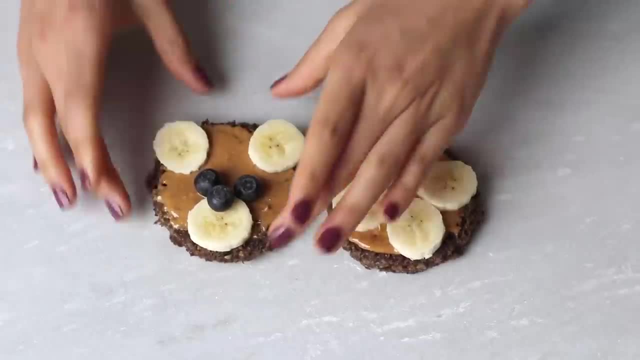 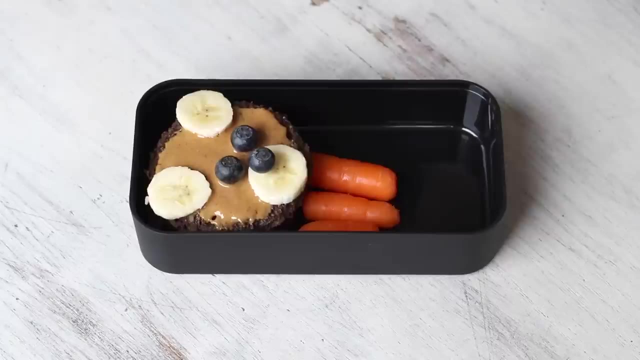 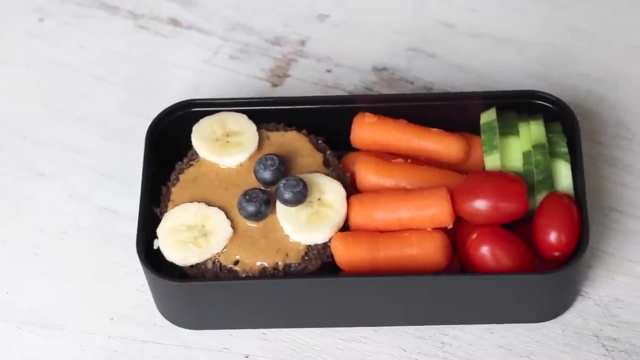 to make an adorable little bear sandwich, Then stack the pieces and place it into the lunch box. I also added some veggies on the side, like baby carrots, cucumber slices and cherry tomatoes To make the cucumbers even more fun for the little. 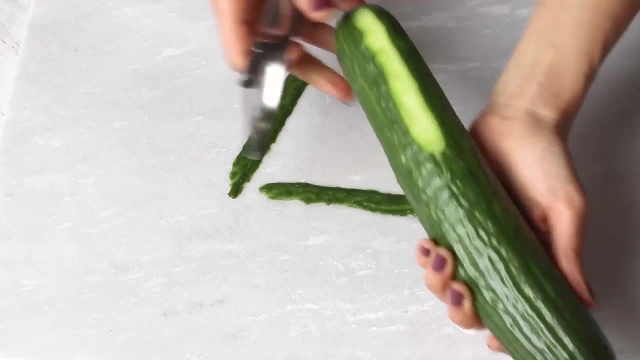 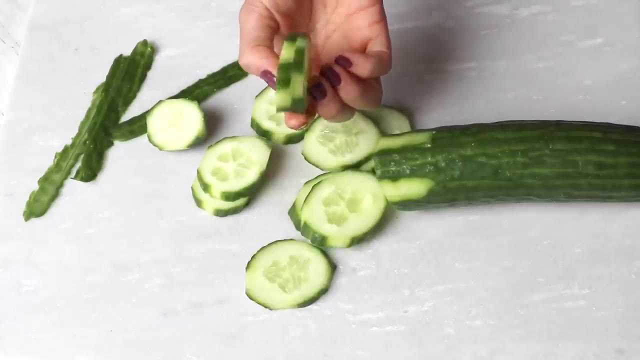 ones to eat. you can peel it as I did before. you cut them up, so that they get this striped pattern Now to make the snacks On the other half of the banana that you didn't use. you can write a message if you'd like. 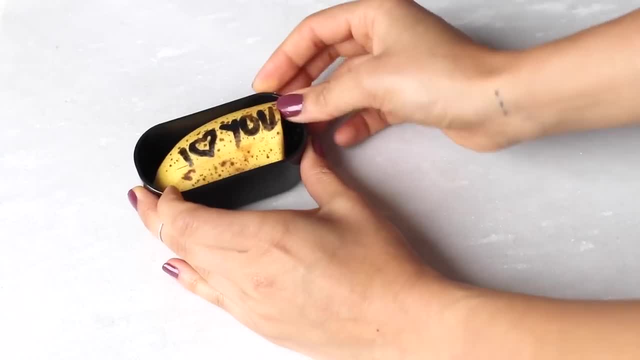 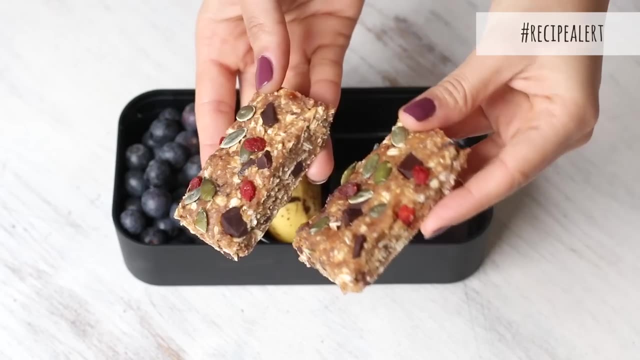 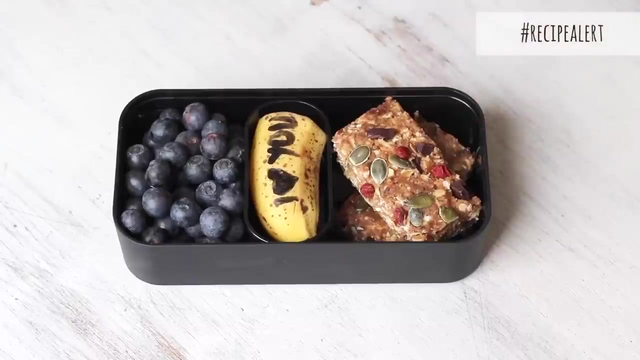 before adding it to the lunchbox. Then I also added some fresh blueberries as well as these chewy peanut butter no-bake granola bars. Like the previous cookie recipe, these are made with only whole food ingredients, so no added sugar or added oil. They too can be made all in the food processor, so very little. 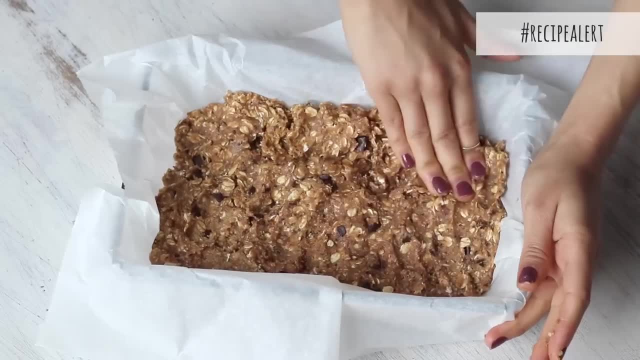 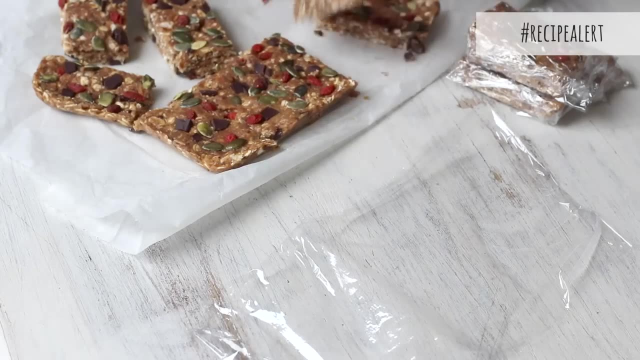 cleaning up required. I also like to make this on the weekends, add different kinds of nuts and dried fruit to keep it interesting each time, and then wrap it up and store it in the freezer so they can be taken as a to-go snack or added. 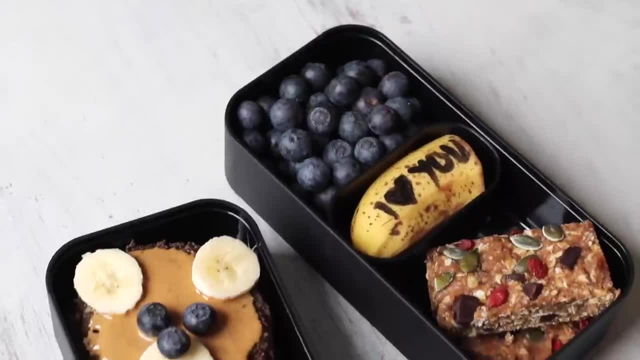 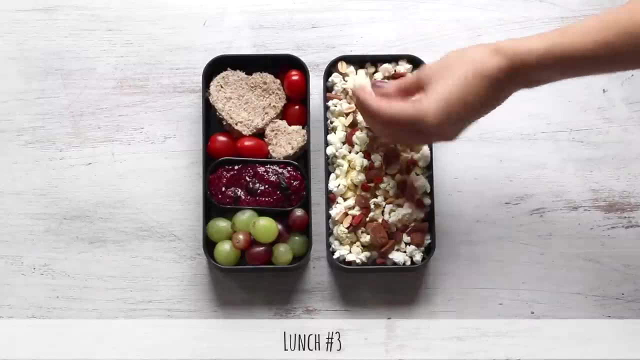 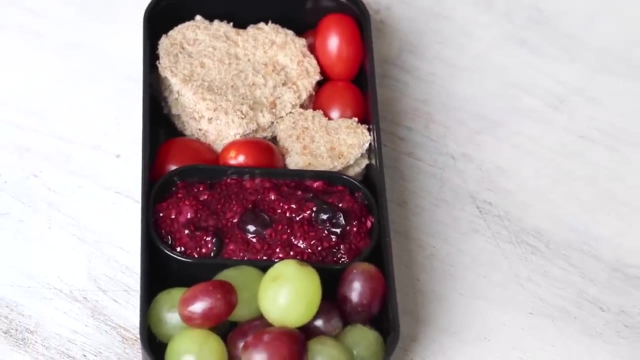 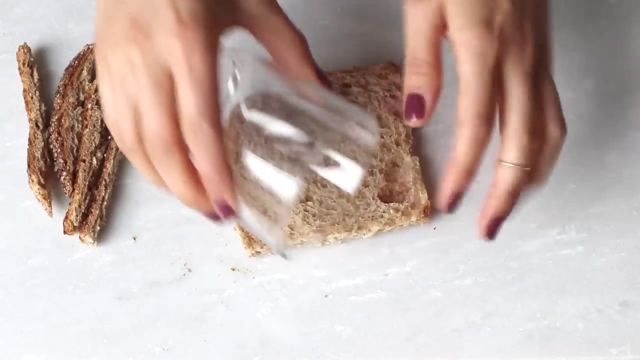 to lunchboxes throughout the week. And that's it for lunchbox number two. And finally, for lunchbox number three, We begin by making this bread and chia jam dip. So first start off by cutting off the crust from a slice of whole grain bread and then roll it out to flatten using either a cup or a. 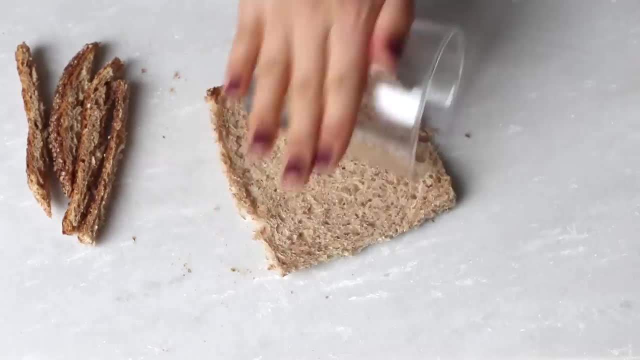 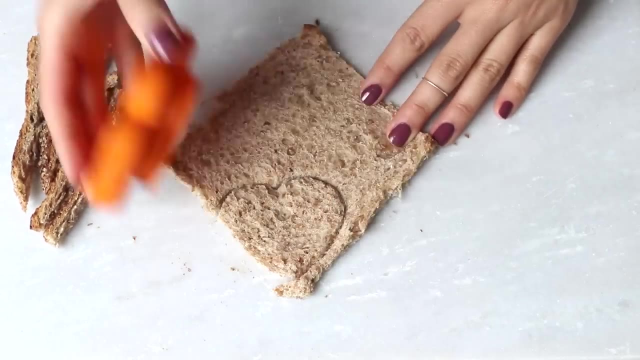 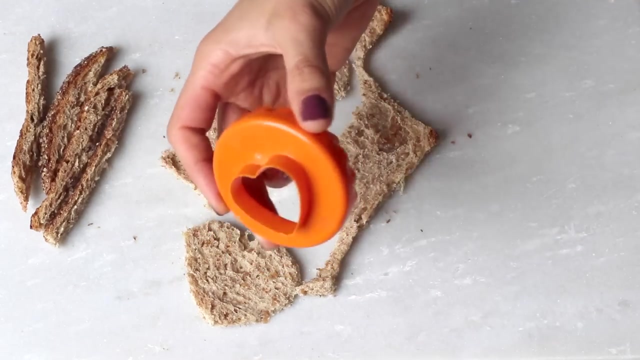 rolling pin, Then cut shapes out of the bread using cookie cutters. I cut out two large hearts as well as two small heart shapes. Now, don't throw away the remaining pieces of bread that you don't use. You can always blend these in a food processor or blender and then freeze. 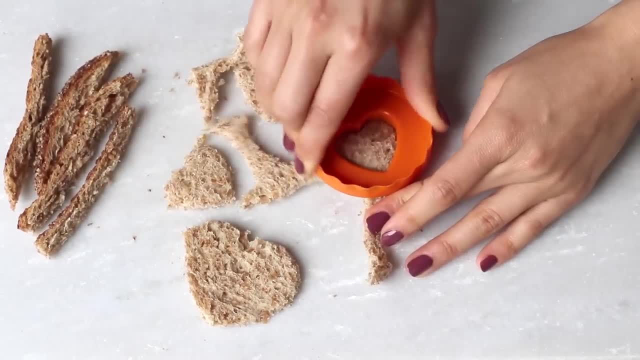 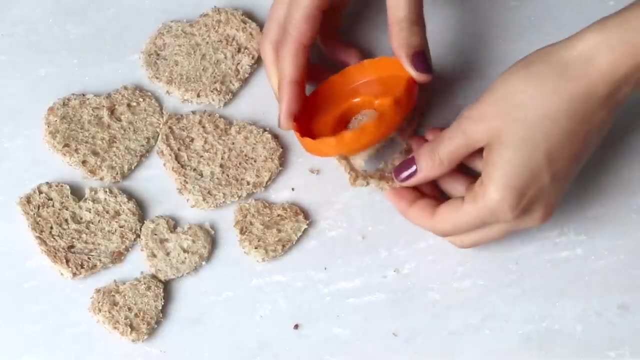 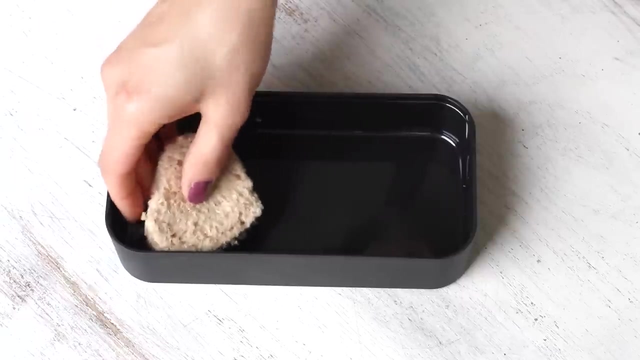 them to use as bread crumbs in future recipes. Then repeat this with another slice of bread. so you end up with four large and four small shapes. of whatever shape you chose. Add this to your lunch box and on the side add some homemade berry chia seed jam. Now this takes. 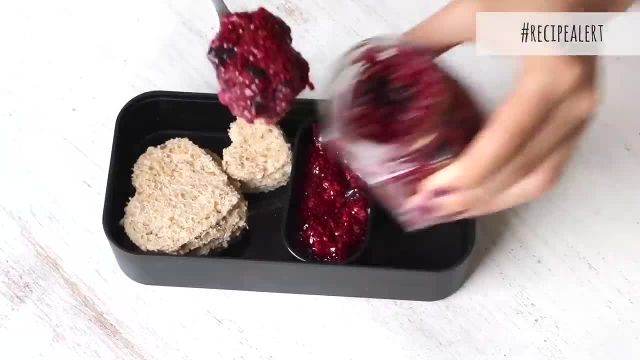 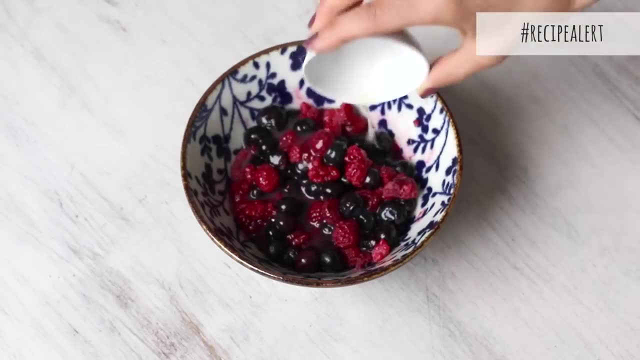 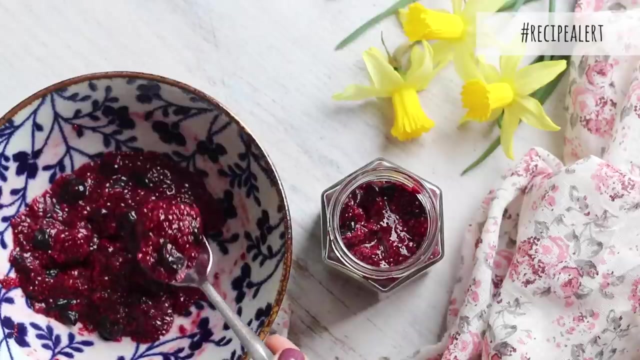 only five minutes to prepare and uses just four ingredients, two of which are different types of berries, and then I also added a little bit of juice and some chia seeds. After you let it sit for 30 minutes, your jam is ready, packed with health benefits: antioxidants, fiber, omega-3 fats. 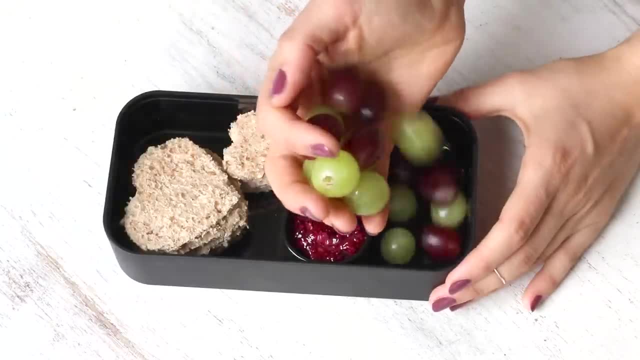 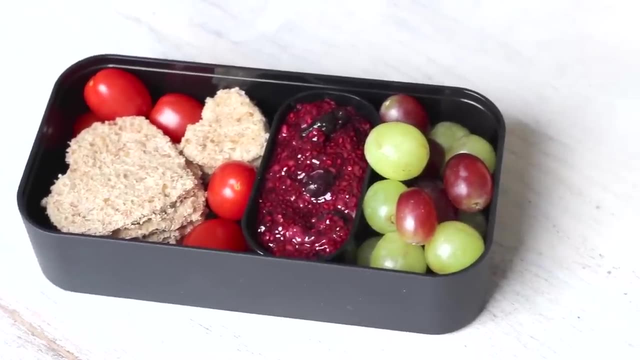 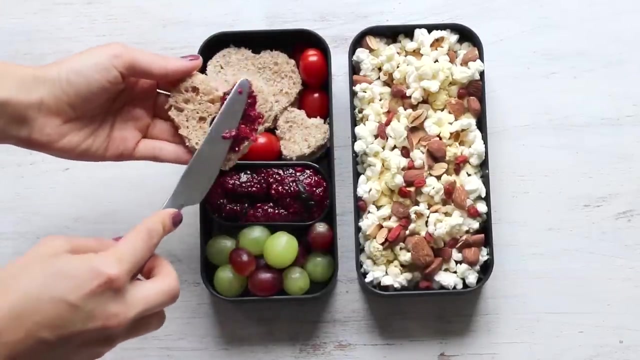 all without any of the added sugar and preservatives that come with store-bought jam. Then on the side I added some fresh grapes and some baby tomatoes To enjoy. your little one can either spread the jam onto the bread, like so, or do a fun dip and dunk. 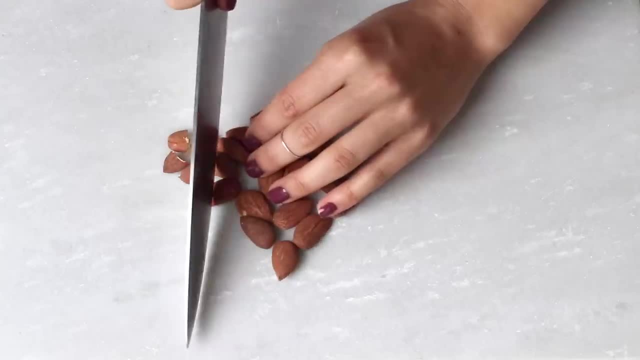 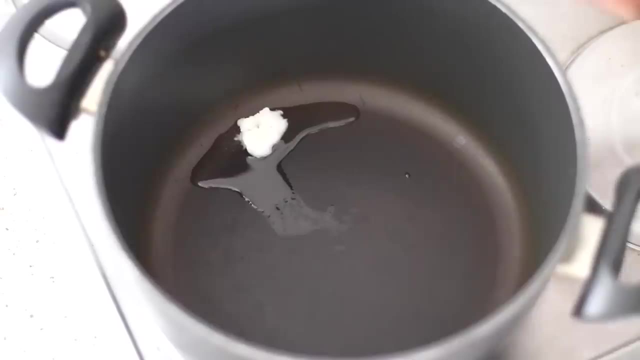 As for the snack on this day, I made this trail mix popcorn. Begin by coarsely chopping some roasted almonds. Then, in a large pot, on medium-high heat, melt about half a teaspoon of coconut oil and add a quarter cup of popcorn kernels and give it a stir. 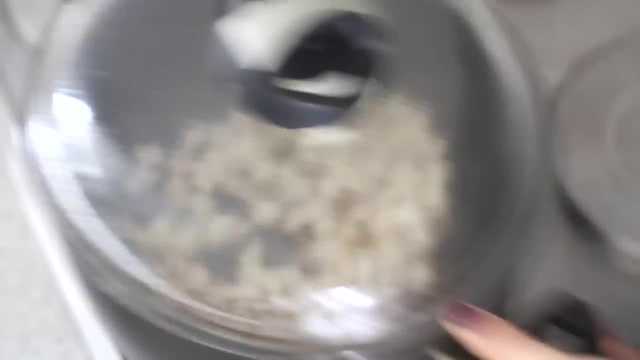 When it starts to pop, shake it periodically so it cooks evenly and doesn't burn. When the popcorn is cooked, you can turn off the heat and let it sit for a few minutes. When the popcorn is cooked, you can turn off the heat and let it sit for a few minutes. When the 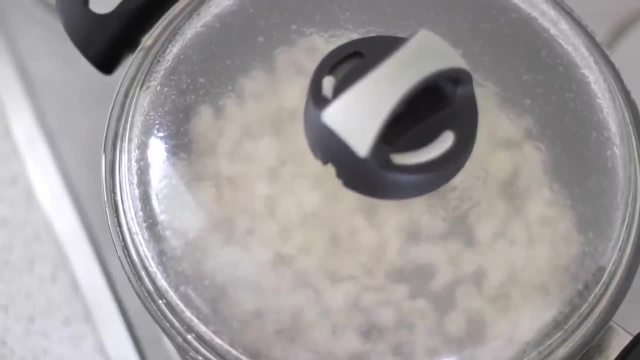 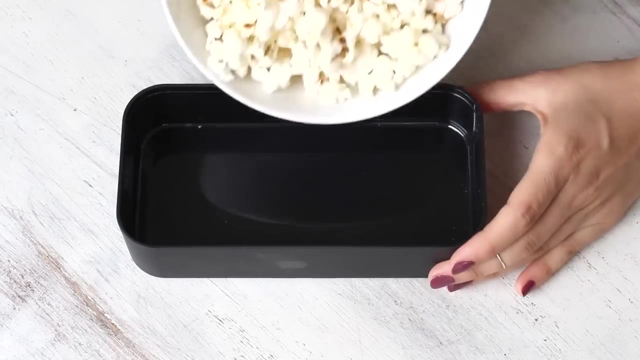 popping quiets down, remove it from the heat. Of course, to speed this up, you can always use butterless microwavable popcorn too. Popcorn is a whole grain source, so it's a great and fun way to get fiber into your little ones. I also added about a teaspoon of nutritional yeast, which gives it a 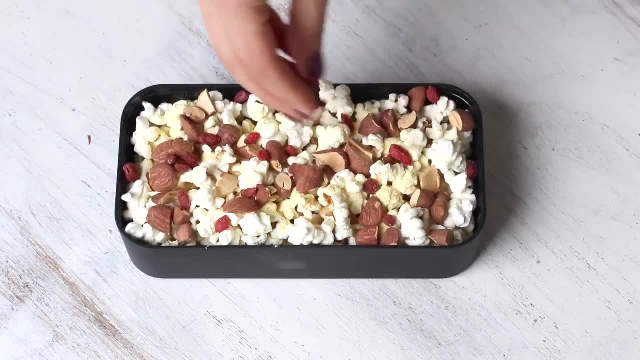 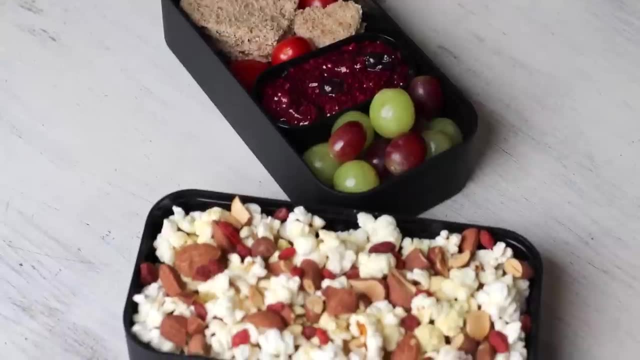 cheesy flavor and also adds vitamin b12. Then you can add the almonds and some goji berries, or use raisins or dried cranberries if you'd like. And that's it for lunchbox number three. Now there's a few things that you can add to your lunchbox. First of all, you want to make sure that you're 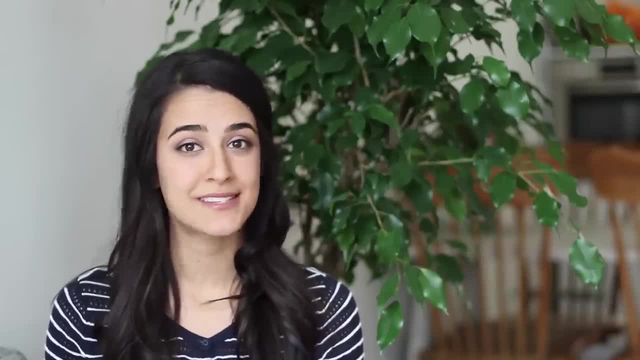 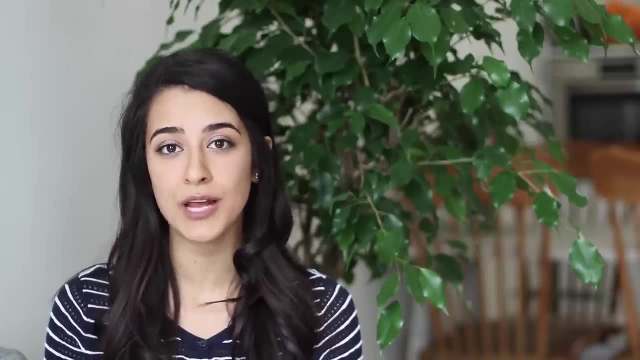 making a lunchbox. You don't need bento boxes to make this. Any lunch container will do. If your kid happens to be quite young, you might want to consider chopping up any choking hazards, like grapes, cherry tomatoes or some of the nuts that I share in these recipes As well. if your kid 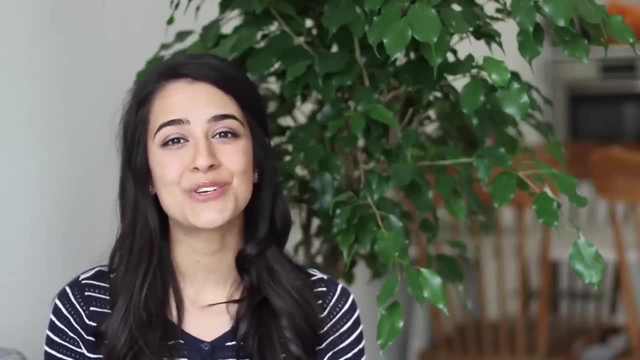 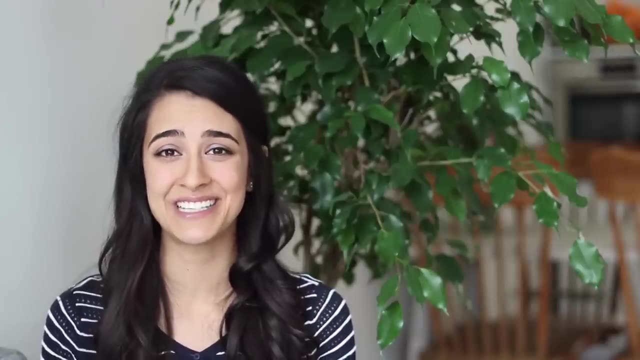 happens to be in a nut-free school, you might want to consider using some kind of nut-free spread like wow butter. anytime I use something like peanut butter. Now, weren't some of those ridiculously adorable? I personally loved making the little bear sandwich. I hope that you've. 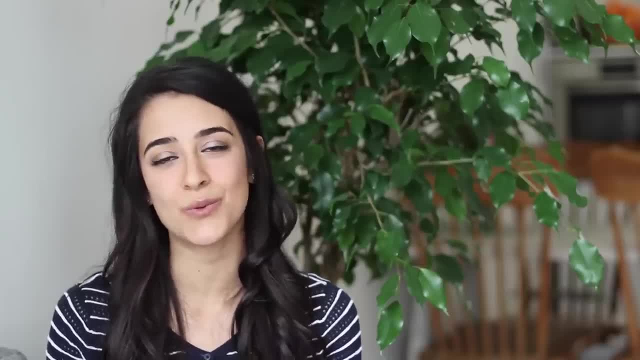 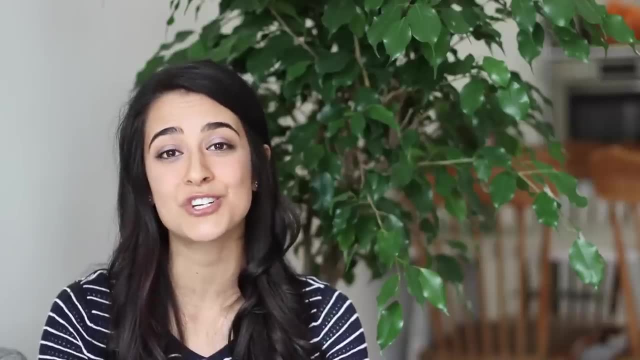 found some ideas and some inspiration and if you want to try any of the recipes, like I said, the link to them can be found in the description box below. If you liked this video, if you found any of the suggestions helpful, share that in the comments below as well. give this video a thumbs up. 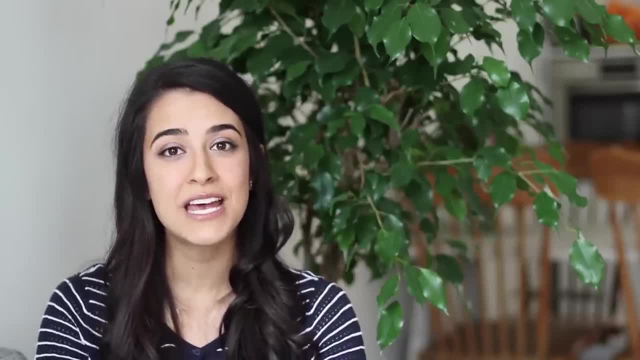 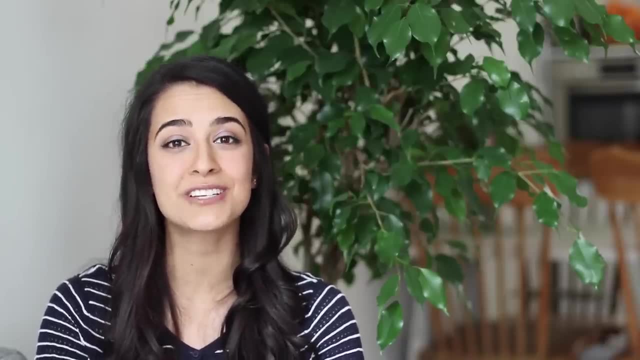 Be sure to also subscribe so you don't miss out on any future videos. and if you want to check out some of the other bento box videos I've made, you can go and check that out on my channel as well. All right, thanks for watching. I'll see you in a few days.